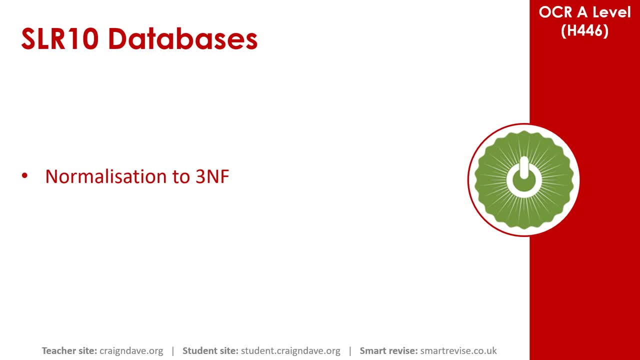 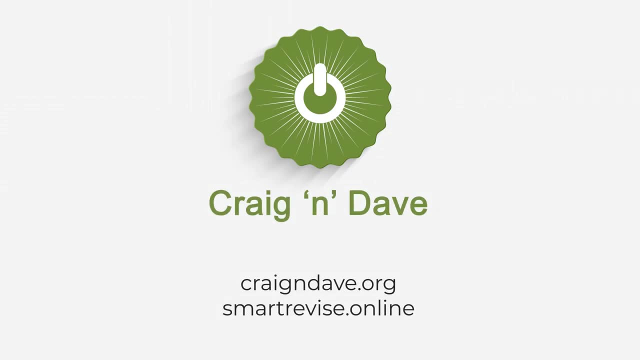 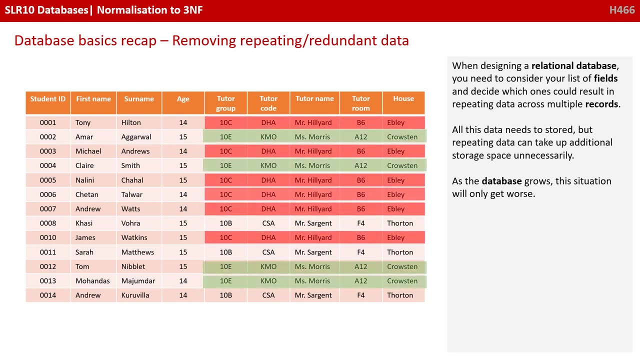 In this video we discuss how to normalize a database to third normal form. Okay, so get ready to buckle in, because this is one of the trickier concepts in the entire A-level specification. So we're going to step through it slowly, bit by bit, with a worked example. 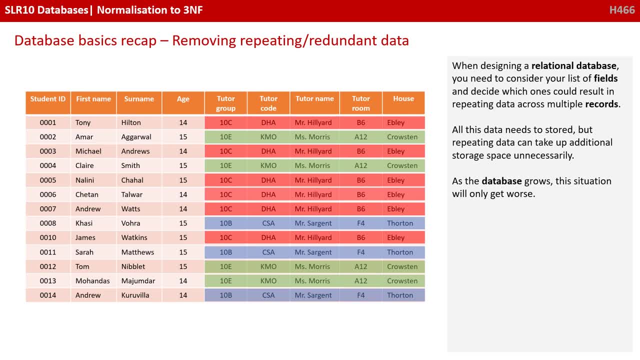 If you don't get it the first time through, we've got an extra video after this which will give another example, and you can re-watch the videos at a later stage. First of all, let's start with a basic recap of some of the fundamentals. When designing a relational database, you need to 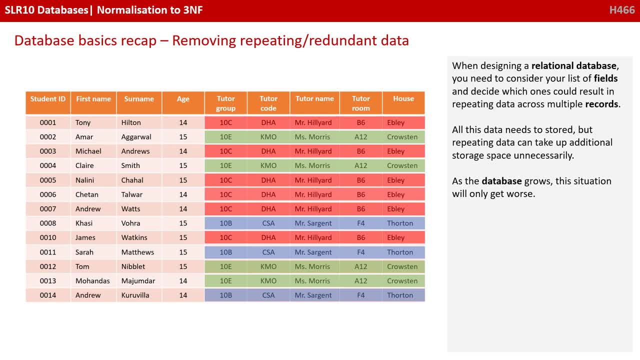 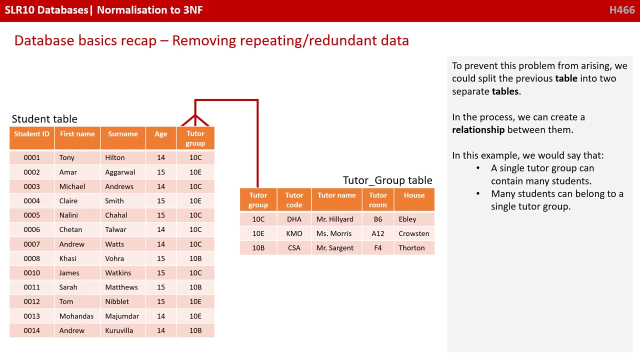 consider your list of fields and decide which ones could result in repeating data across multiple records. All this data needs to be stored, but repeating data can take up additional storage space unnecessarily. As the database grows, the situation will only get worse. To prevent this problem from arising, we can split the previous table into two tables In the process. 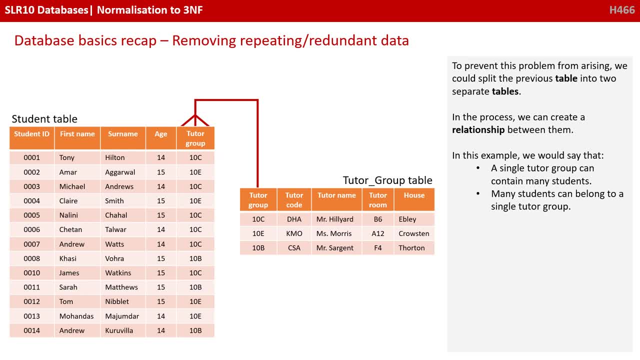 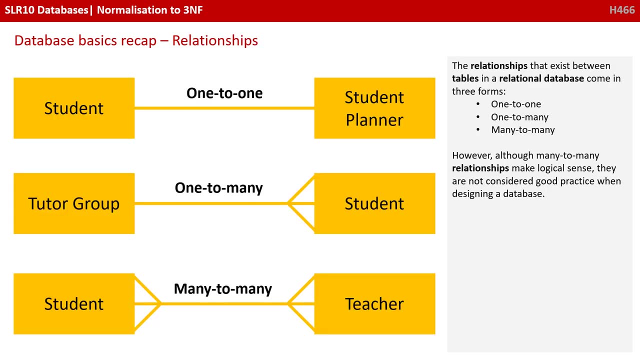 we create a relationship between them. Here we say that a single tutor group can contain many students or that many students can belong to a single tutor group. The relationships that exist between tables in a relational database come in three formats: one-to-one, one-to-many. 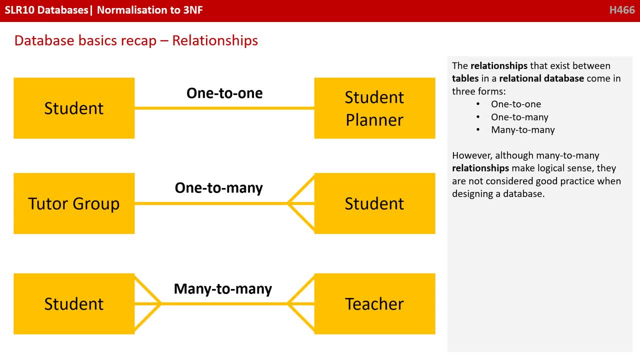 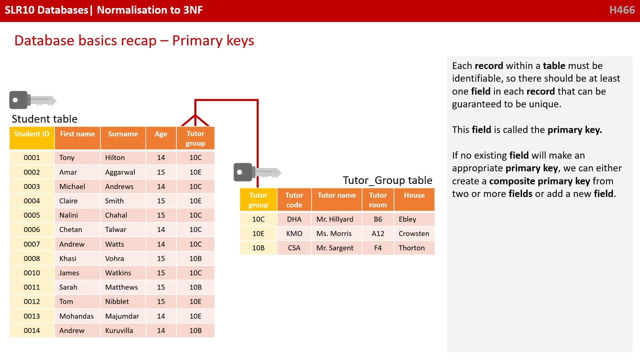 However, although many-to-many relationships make logical sense, they are not considered good practice when designing a database. Each record within a table must be identifiable, so there should be at least one field in each record that can be guaranteed to be unique, and this field we call the primary key. 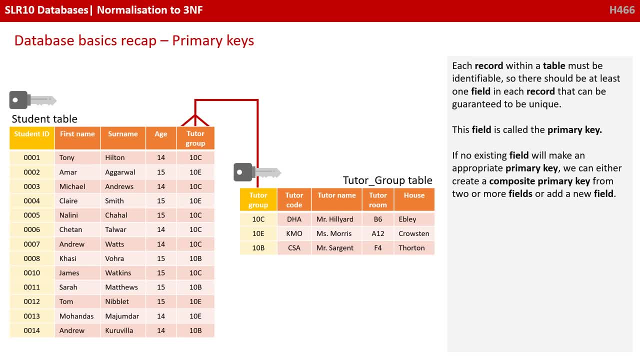 If no existing field will make an appropriate primary key, we can either create a new primary key or create a new primary key. We can use a composite primary key from two or more fields or simply add a brand new field that we make our primary key. 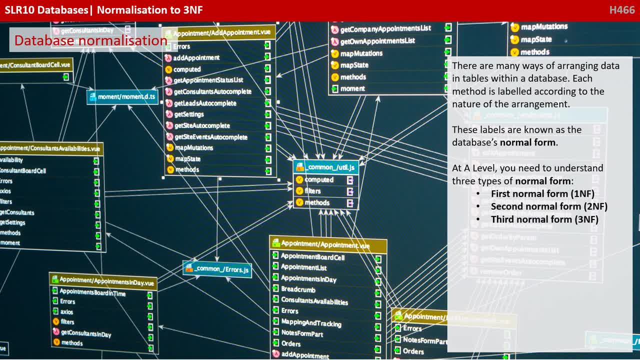 Okay, so that's the recap. let's actually look now at database normalization. So there are many ways of arranging data in tables or in a database, and each method is labeled according to the nature of this arrangement. These labels are known as the database normalization. 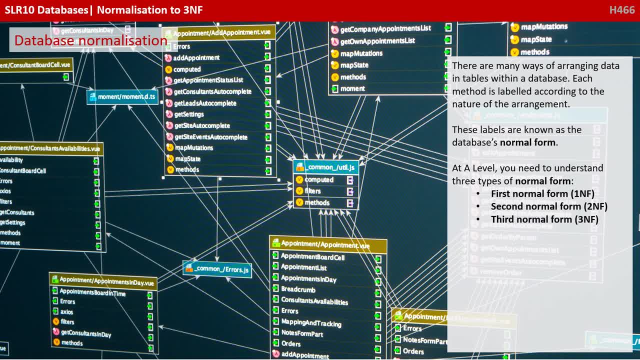 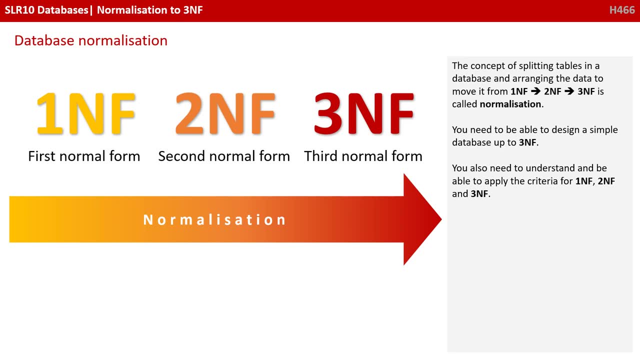 So let's take a look at one of the most common ways of arranging data in a database At A level. you need to understand three types of normal form: first, second and third normal form- The concept of splitting tables in a database and arranging the data to move it from. first. 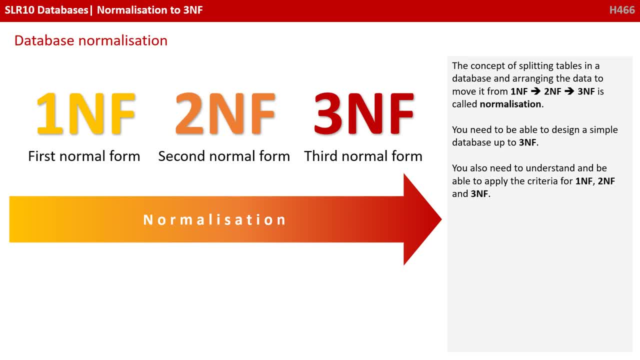 second and into third normal form is the process of normalization. You need to be able to design a simple database up to third normal form. You also need to understand the criteria and be able to apply the criteria for first, second and third normal form. 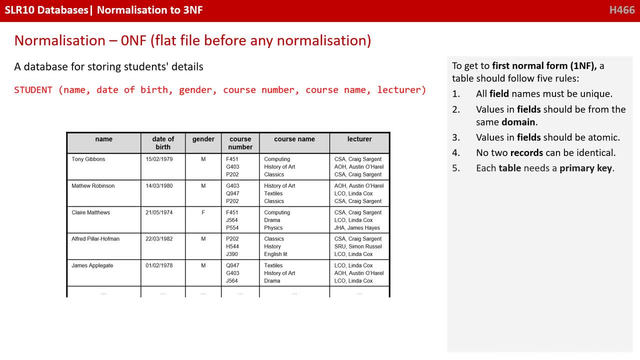 Okay, so let's start with an unnormalized database, sometimes referred to as zero and F or UNF, unnormalized. You can see, here we just have a table that's got everything in it. To get us to first normal form, a table should follow five rules. 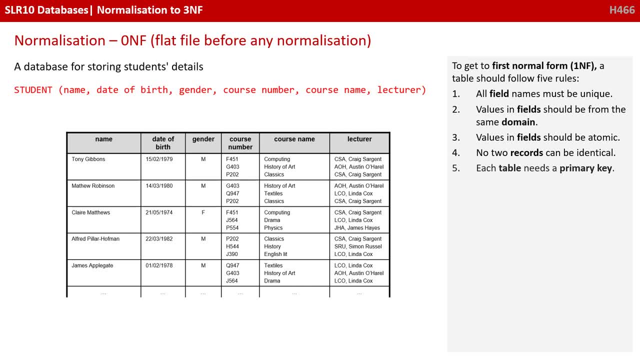 All field names should be unique, values and fields should be from the same domain. values and fields should be atomic. no two records can be identical and each table needs a primary key. Now let's work through these and explain what they mean and apply it to our unnormalized table of. 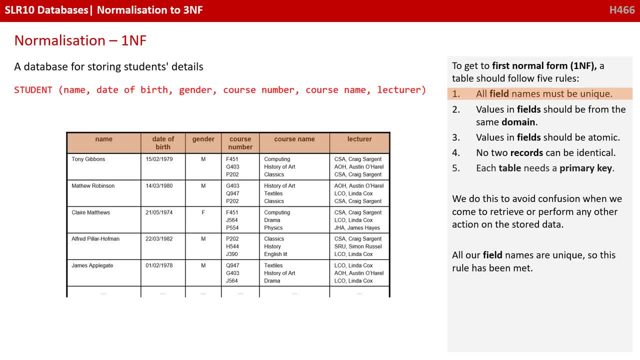 data. So, first of all, all fields must be unique. Well, we simply do this to avoid confusion. it's pretty much common sense. When we come to retrieve or perform any sort of action on the stored data, if the field names aren't unique and are replicated, it's going to become very confusing. 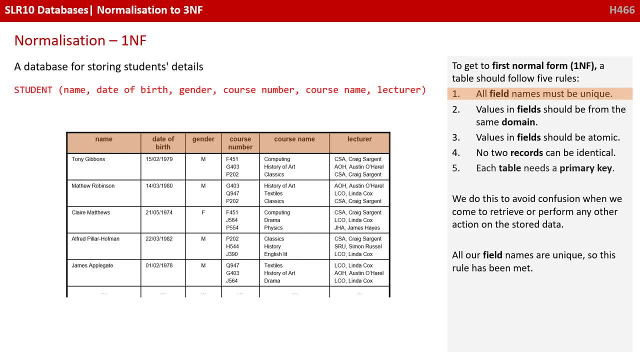 Now all our field names are unique here: name, data, birth, gender, course, number, course, name, lecturer. so this rule has already been met. Rule 2: values and fields should be from an unnormalized database, the same domain. So what we're saying is: in each field, the stored values must be. 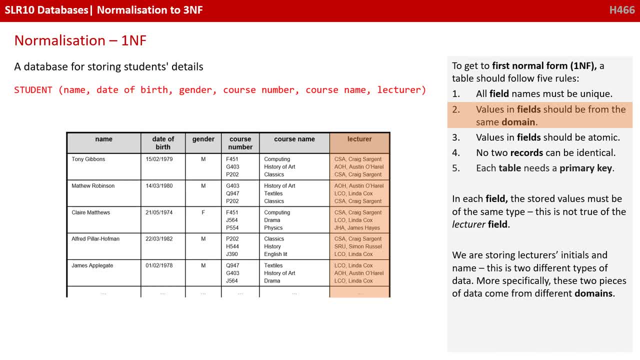 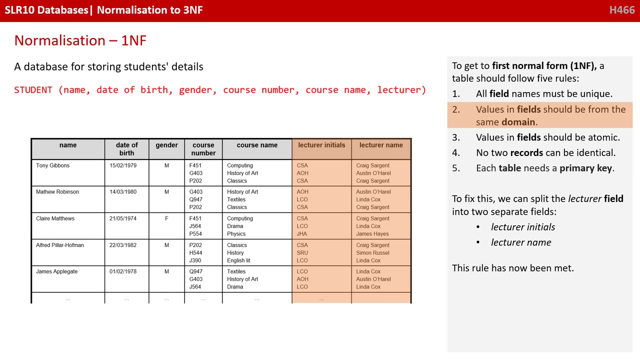 of the same type. Well, this isn't true of the lecturer field. We're storing the lecturer's initials and we're also storing their name. This is two different types of data. More specifically, these two pieces of data come from different domains, So we haven't met rule 2.. The fix is simple: We split that lecturer. 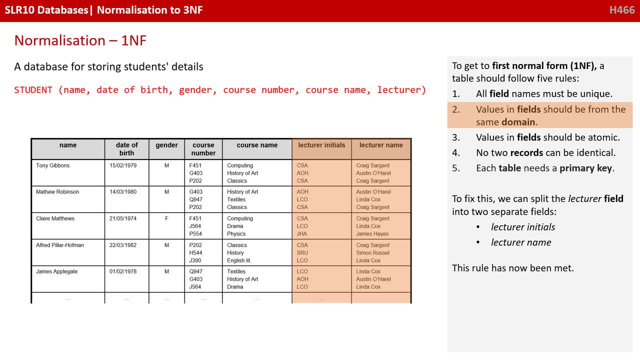 field into lecturer initials and lecturer name. Now rule 2 has been met. Rule 3 says values and fields should be atomic. So for every record and field intersection, in other words for every kind of square or cell on this table, we should only have a single value. Now we can see that the fields course number. 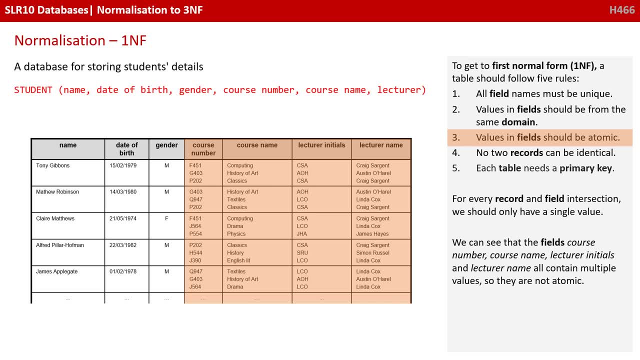 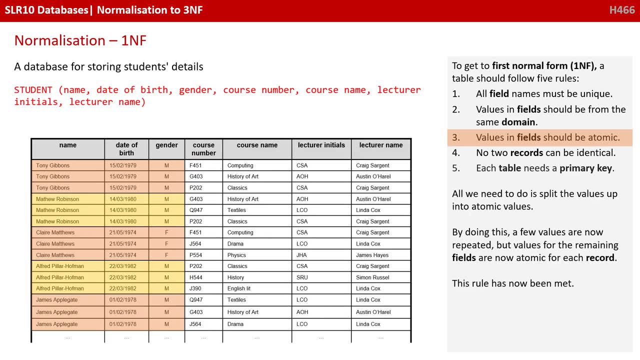 course, name, collateral initials and lateral names all contain multiple values, So these are not atomic. So currently we're failing on rule 3.. All you need to do is split the values up into atomic values. By doing this, a few values you can see. 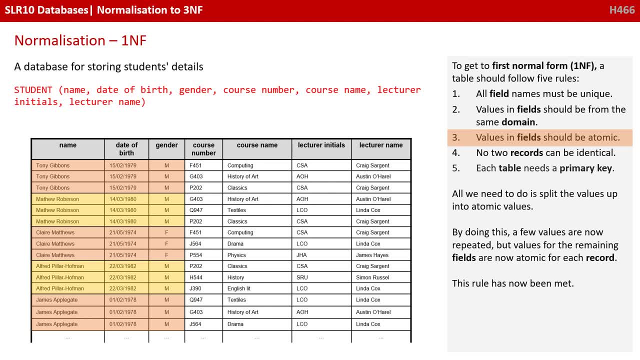 have now become repeated. but values are stories. So if Iضl, oktwo values and corresponding values, then all the fields areräge with mortal values or values with, for the remaining fields are now all atomic for each record. so this rule has now been met. now at 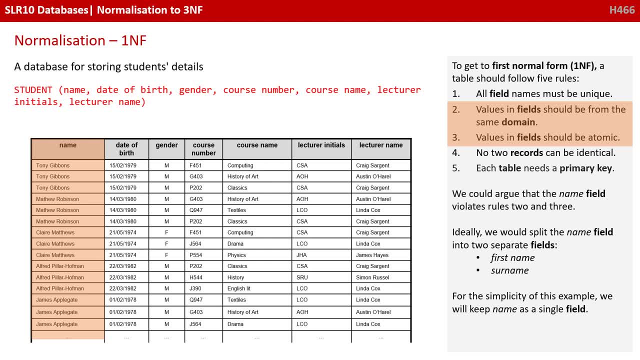 this point, if you've been paying attention, you could argue that the name field violates rules two or three. you can say: well, they're not really atomic, are they? and they're holding two different types of data: a first name and a surname. now, ideally, we would split the name field into two. 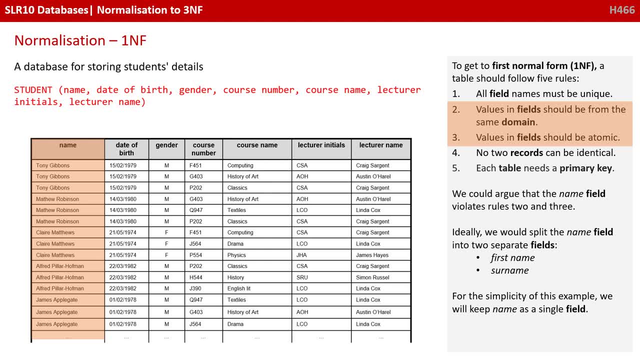 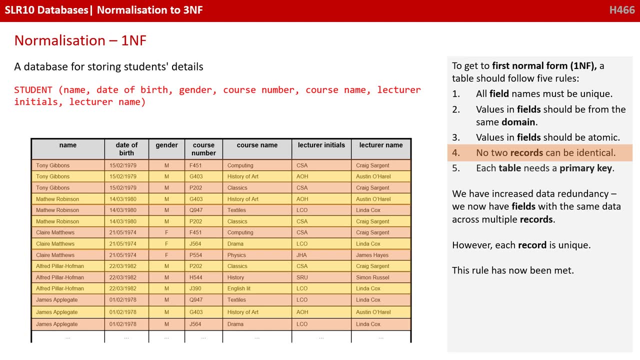 separate fields. first, name and surname. for pure simplicity, and for this example, we're just going to keep name as a single field. but if you spotted that, well done. so on to rule four: no two records can be identical. now we've massively increased data redundancy here. we now have fields with the 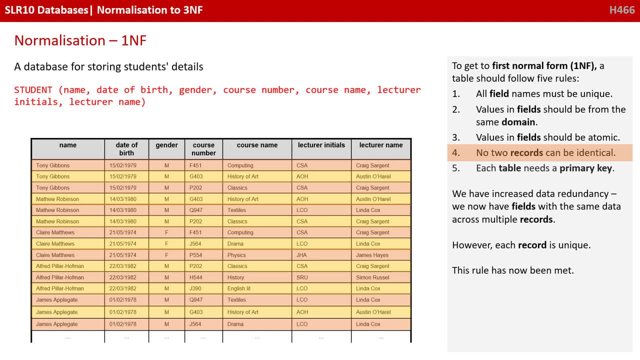 same data across multiple records. however, each record is completely unique, so rule four is unique. so rule four is completely unique. so rule four is completely unique. so rule four is unique. so rule four is completely unique. so rule four is completely unique. so rule four is completely Transceksin. 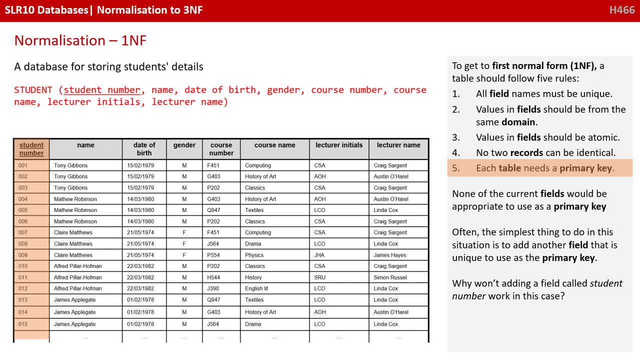 finally, each table needs a primary key. now, none of the current fields would be appropriate to use as a primary key. they could all be repeated often. the simplest thing to do in this situation is to add another field that is unique to use as a primary key. now I've done that here, but 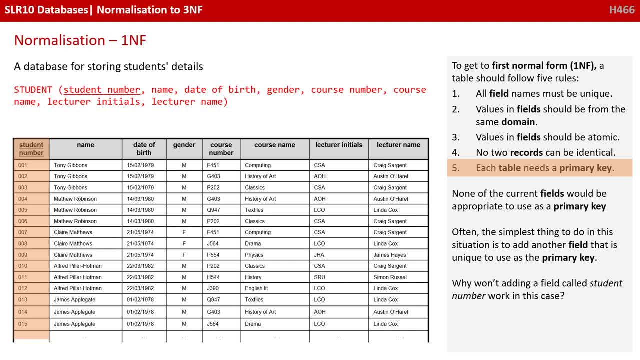 have a quick look. why won't adding a field called student number work in this case? well, although it looks like having added the student number field, each record now has a primary key. it is. each row has a separate unique number. each student now has three different student numbers. so Tony Gibson is student 1, 2 & 3, so that's. 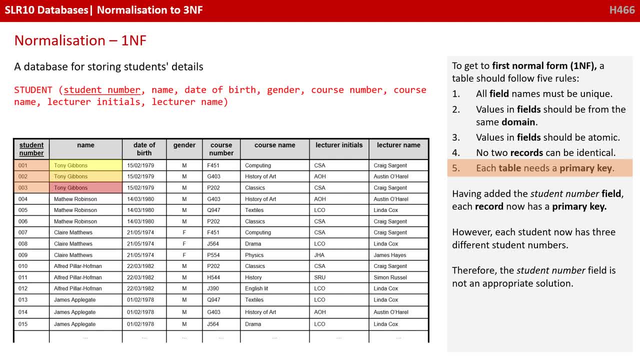 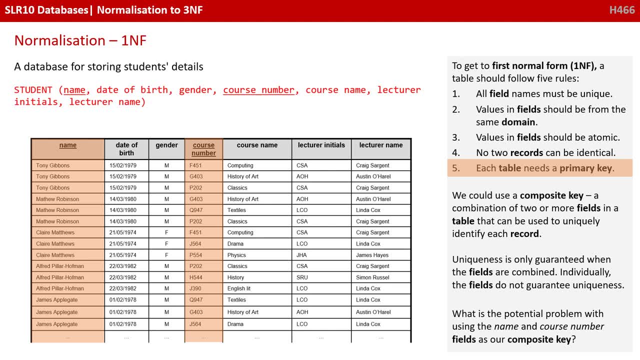 not working. the student number field is really not an appropriate solution. we could use here what's known as a composite key, a combination of two or more fields in a table that can be used to uniquely identify each record. now, uniqueness is only guaranteed when the fields are combined individually. the 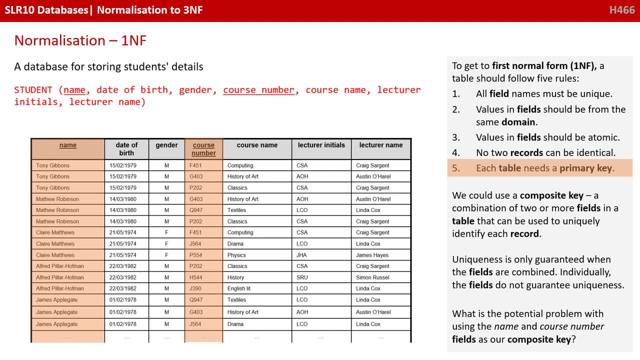 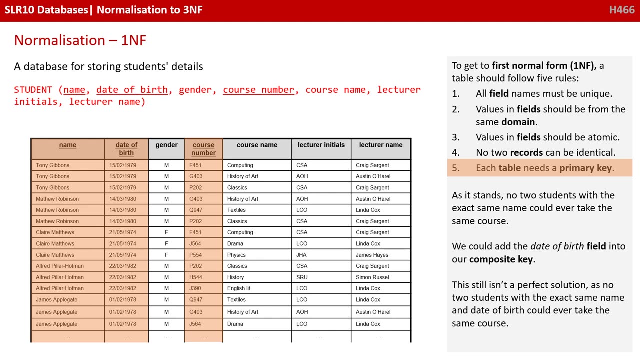 fields do not guarantee uniqueness, and this is what makes it a composite primary key. so what could be the potential problem with using name and course number fields together as our composite primary key? well, as it stands now, if we did that, no two students with the exact same name could ever take the same course, because we 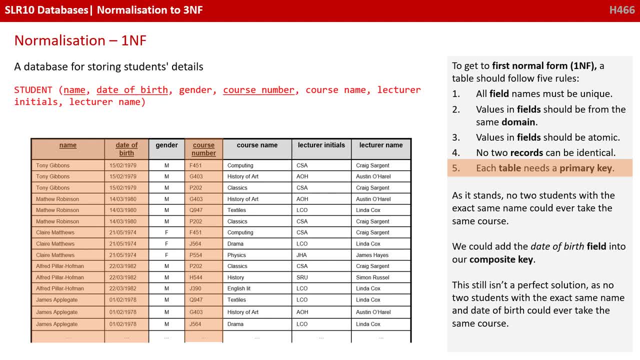 can't have repetition in the primary key, we could decide to add the date of birth field, so now we've got three fields together, making our composite key. now, this isn't a perfect solution either. that's what we're saying now is no two students with the exact same name and 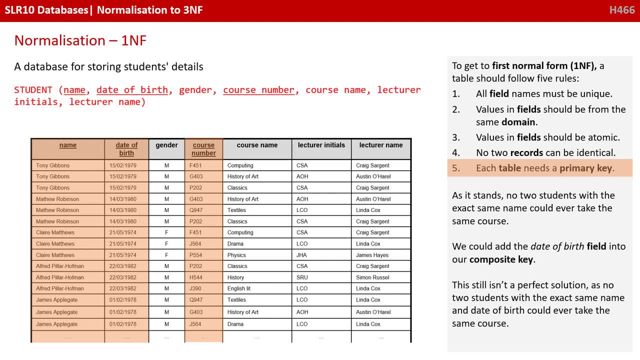 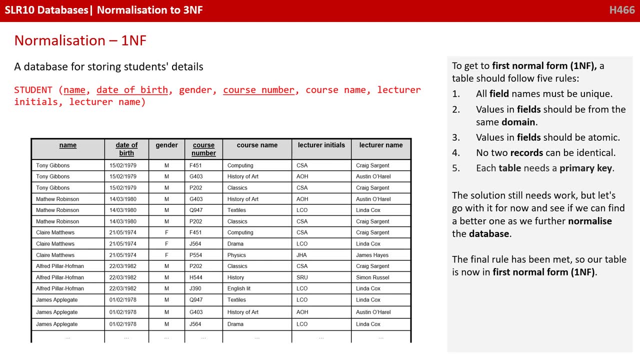 date of birth could ever take the same course. now you could argue this is highly unlikely and this is a. this is a good solution for our composite primary key, but it feels a little messy. this solution clearly still needs some work, but let's go with it for now and see if we can find a better one as we further. 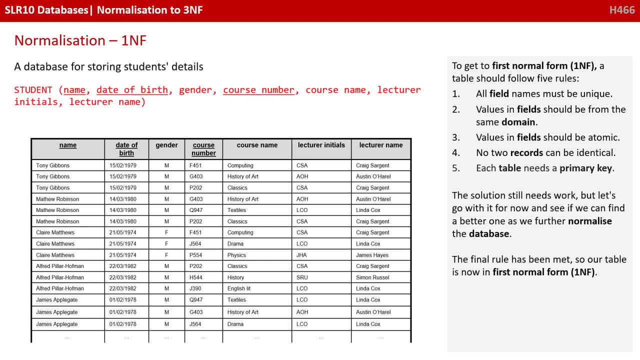 normalize the database for point. however, we'll go to the next slide and see if we can find a better one as we further normalize the database. the point, however, as we further normalize the database. the point, however, is the final rule has now been met. so all five rules have been met, so our table is: 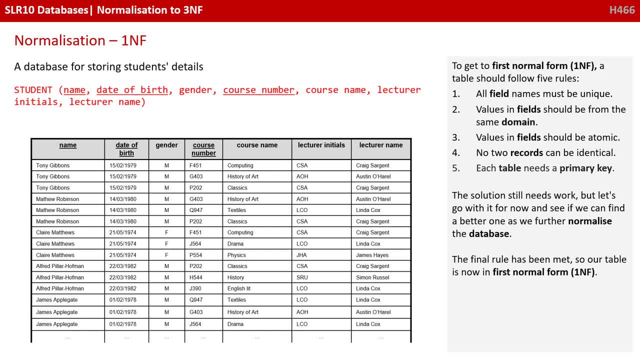 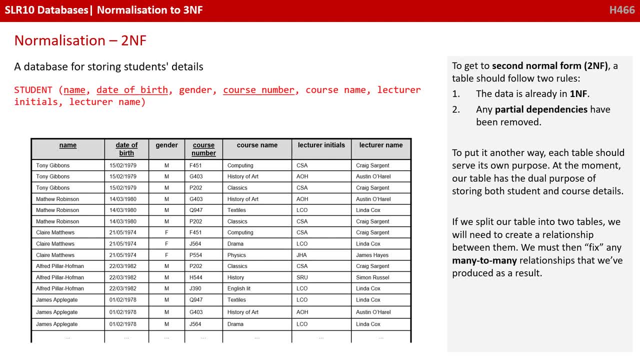 now in first normal form. So to get to second normal form, you'll be pleased to hear there's a lot less rules to follow. You have to follow two: Make sure the data is already in first normal form and make sure any partial dependencies have. 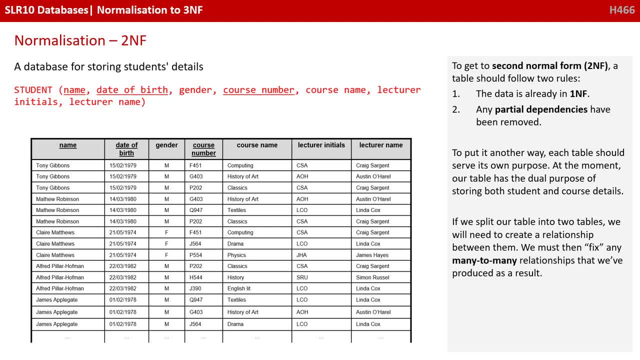 been removed. So what I mean by that? well, to put it another way, we're trying to make sure here that each table serves its own purpose. At the moment, our table has a dual purpose of storing both the student and all of the associated course. 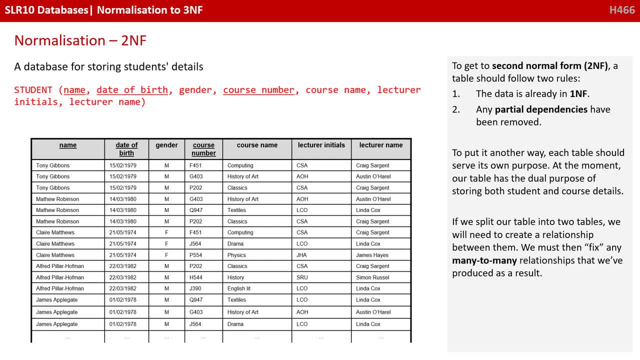 details. If we split our table into two tables, we'll need to create a relationship between them and remember we must fix any many-to-many relationships that we produce as a result of this. So, if we split our table into two tables, we'll need to create a relationship between them and remember we must fix any many-to-many relationships that we produce as a result of this. So if we split our table into two tables, we'll need to create a relationship between them and remember we must fix any many-to-many relationships that we produce as a result of this. So if we split our table into two tables, we'll need to create a relationship between them and remember we must fix any many-to-many relationships that we produce as a result of this. 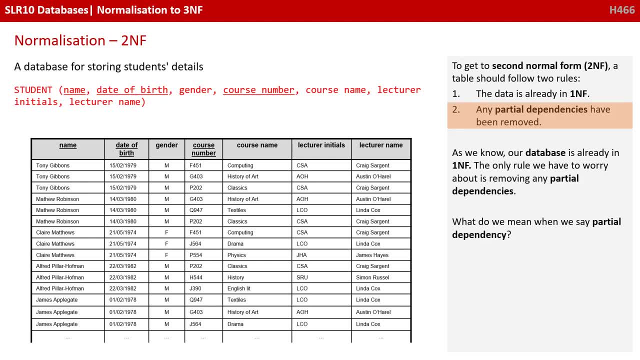 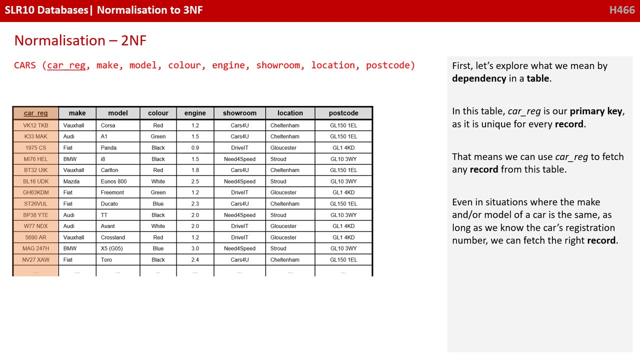 So we know our tables already in first normal form. so let's deal with the second rule: Make sure any partial dependencies have been removed. So what do we actually mean by this partial dependency? Well, let's take a step back, because it's really important you get your head around this. So first let's 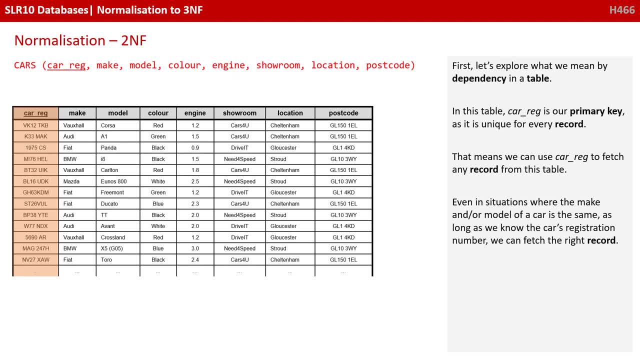 explore what we mean by dependency in a table. So here we've got a table storing car details. In this table, car reg is our primary key. It's unique for every record. That means we can use car reg to fetch any record from this table, Even in situations when the make and model of 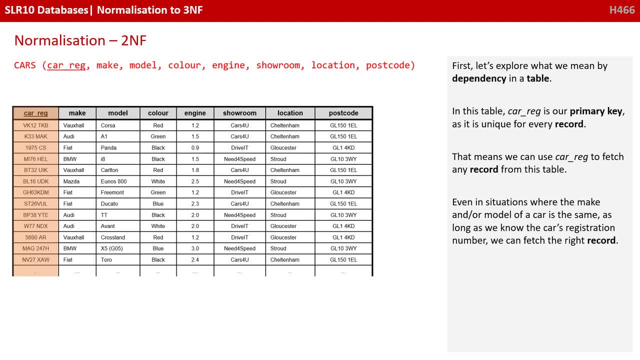 the car is the same. as long as we know the car's registration number, we can fetch the right record. For example, I can ask for the model of car, reg BL 16 UDK, and I will get the answer. I can ask for the color of cars. 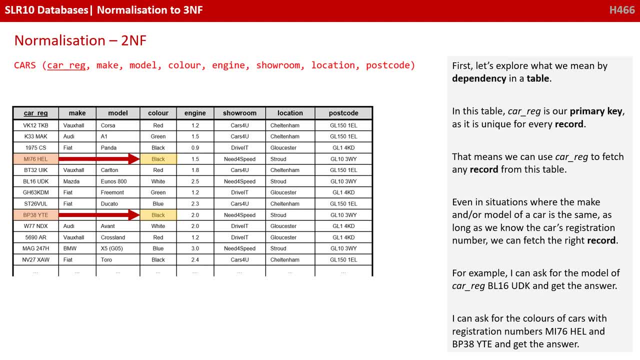 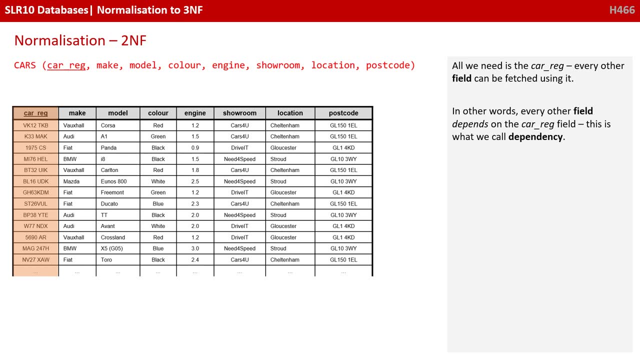 with the registrations M176HEL and BP38YTE and I will get the answer. All we need is the car reg. Every other field can be fetched using it. In other words, every other field can be fetched. Every other field depends on the car wedge field. 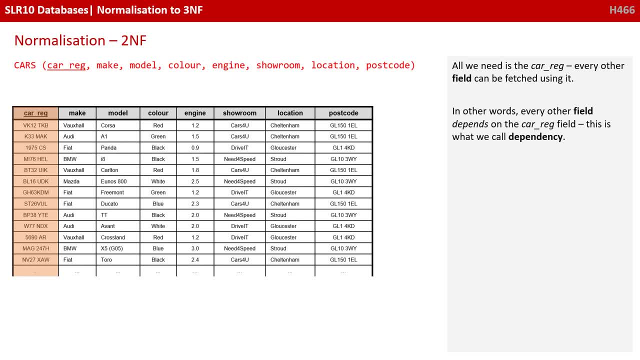 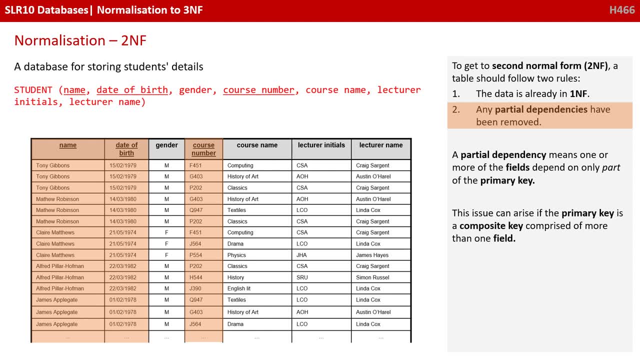 And this is what we call dependency. Now, a partial dependency means that one or more of the fields depend on only part of the primary key, And this issue can arise if the primary key is a composite made up of more than one field, which is what we've got here. 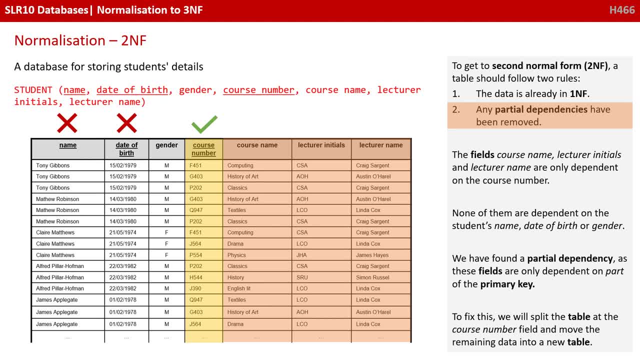 The field, course name, lecturer initials and lecturer's name are only dependent on the particular course they're taking, the course number. None of those fields are dependent on the student's name, date of birth or gender. that is kind of irrelevant. 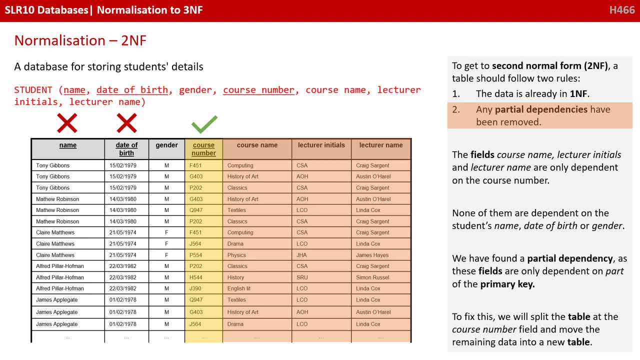 So we found a partial dependency, as these three fields are only dependent on both the primary key and the secondary key. So Part of the primary key, the course number field. So to fix this, we'll split the table at the course number field and move the remaining data into a brand new table. 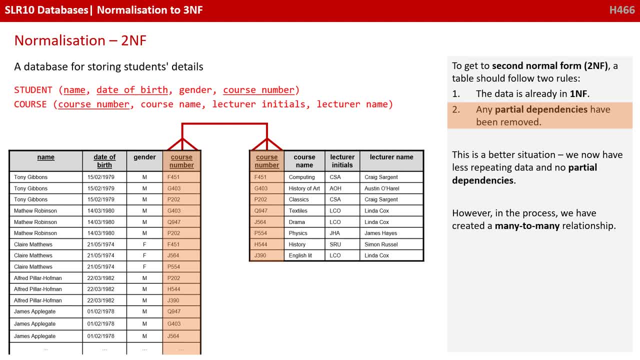 Now this is a much better situation. We now have less repeating data and we've got no partial dependencies. However, in the process, we have created a many to many relationship. We're saying here a student should be, Let's take many courses and of course can have many students and remember. although that makes logical sense, databases don't like many to many relationships. we have to fix that somehow. 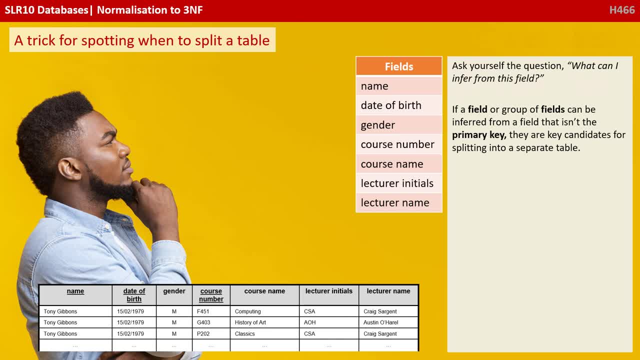 Now I'm just gonna take a quick step back. This Trick of spotting when to split a table to go to first to second normal form can often cause a bit of confusion when you first start to do it Now. after a bit of practice it will become really easy. 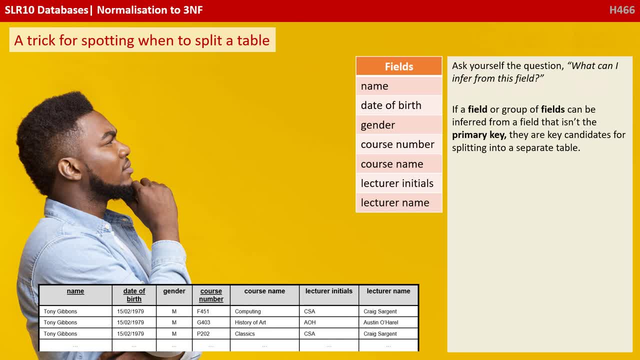 You'll spot it quickly. but while you're learning the process, here's a quick trick. when you're looking to split that table up, ask yourself the question: what can I infer from this field? What can I work out or determine from this field? 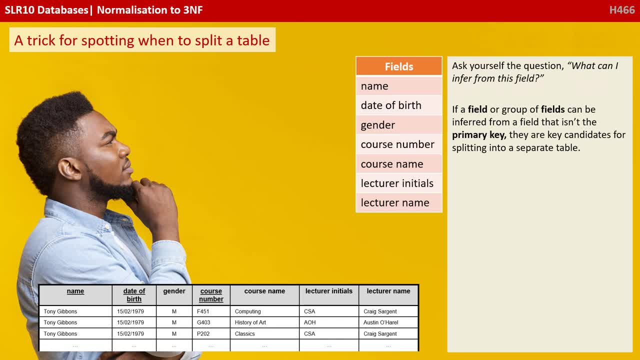 If a field or group of fields can be inferred from a field that isn't the whole primary key, then they are key candidates for splitting into a separate table. So let's try. Let's look at the name field. Ask yourself, if I know a student is called Tony Gibbons. can I infer anything from that? 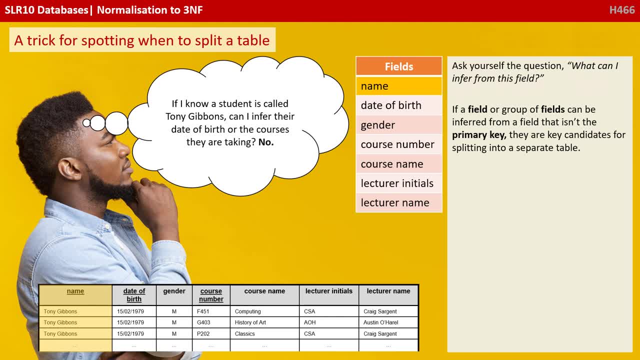 Just because you're told Tony, can I infer their date of birth? Can I infer the course someone would take just by their name? No, I can't. Okay, let's move on. If I know, a student is born on the 15th of the second 1979.. 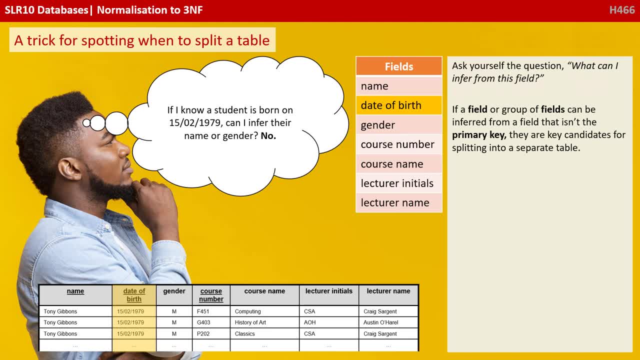 Can I therefore infer? Can I infer their name or gender? No, of course I can't move on. If I knew, if I know a student is male, can I therefore infirm or know automatically their name or what course? No, of course I can't. 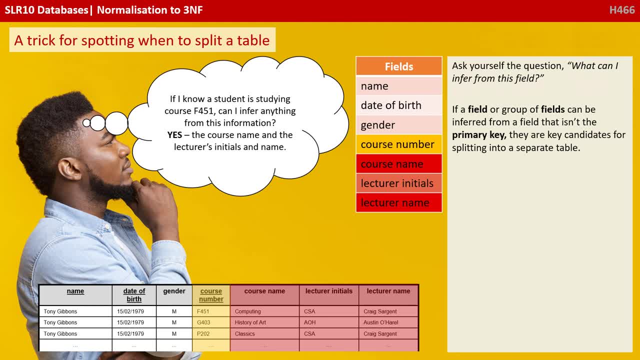 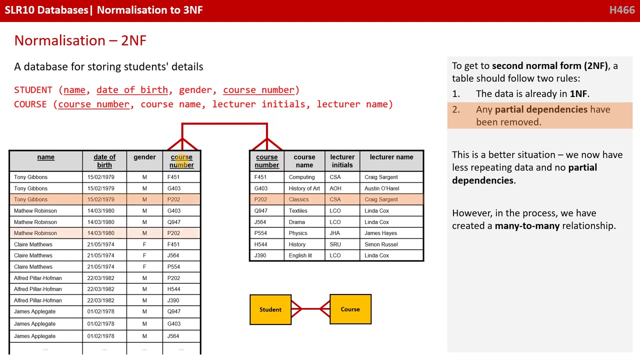 If I know a student is studying course F451, can I infer anything from that? Yes, If they're studying F451.. I know, Of course it's gonna be computing and their lecture is going to be CSA, Craig Sargent. Okay, so there was that little trick. now we can see here we've got a better situation. 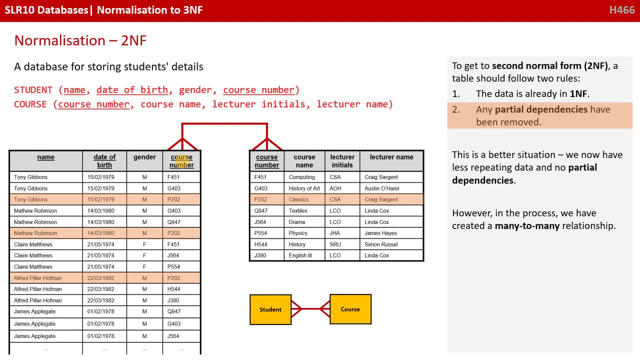 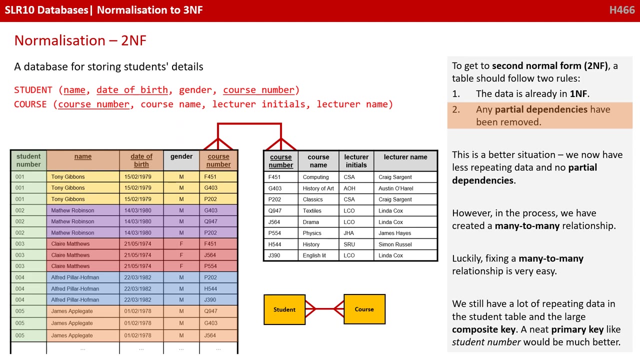 We now have less repeating data, as I said before, but we've created this many, two many relationship which we need to deal with somehow. Luckily, Fixing a many-to-many relationship is very easy. We still have a lot of repeating data in this student table, if you remember, and that happened when we had to meet all the rules of first normal form. 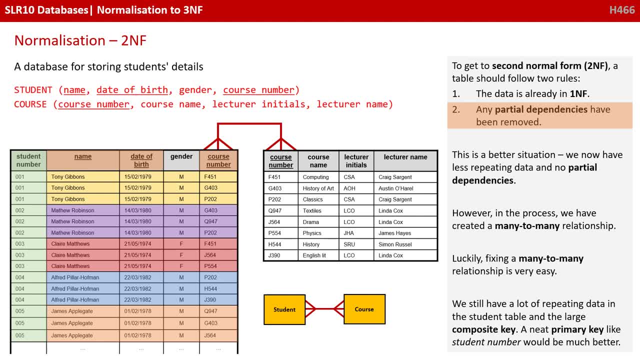 And we also have this really large composite key made of three fields. We'd much rather have a neat primary key like student number. Well, what you're going to discover here is, when we fix this many-to-many relationship, we solve all these issues. 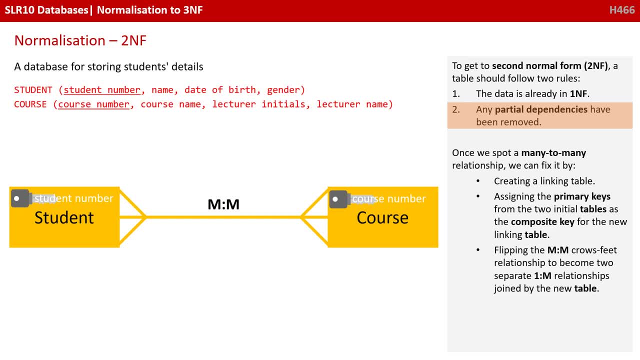 So once we spot a many-to-many relationship, we can fix it by creating a linking table. We assign the primary keys from the two initial tables as a composite key For the new linking table And we flip the many-to-many crow's feet relationships to become two one-to-many relationships joined by the new table. 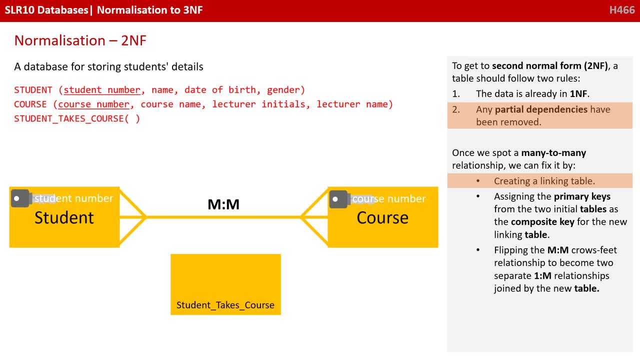 So we create a linking table. We need to give it a name. So this is the table that's going to allow students to take a course. I'll just call it Student Takes Course. We assign it the primary keys of both the tables from either side. 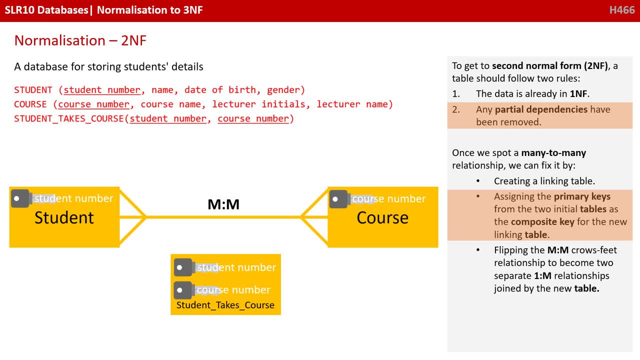 And together they make the composite primary key for our new table. And we flip the crow's feet. We've broken the many-to-many relationship. We flip them and we make two one-to-many relationships And that is the simplest way for you to remember how to deal with a many-to-many relationship. 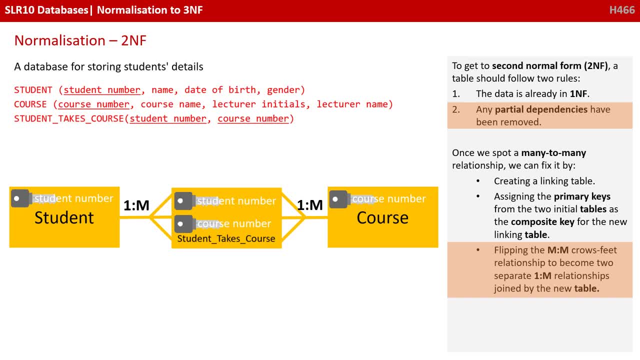 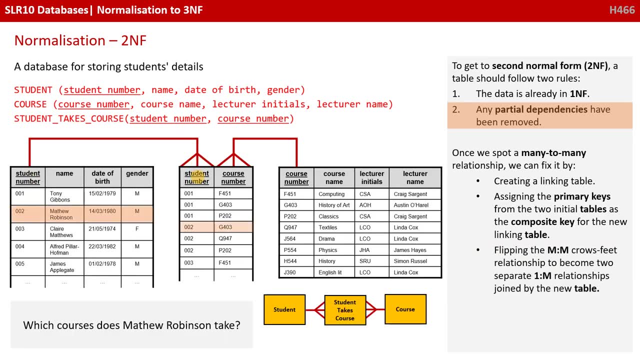 Follow those simple steps. OK, so let's actually have a look at how this works. Which course does Matthew Robinson take? Well, look how easy that was. We've now only got one entry for Matthew Robinson in the student table. We've got rid of three rows for Matthew Robinson. 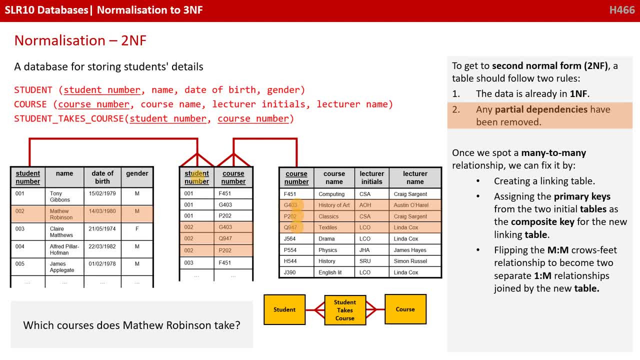 We've got rid of that composite key And now we've managed to put student number in, Because there is one Tony one, Matthew one, Charlie, Matthew Robinson can take multiple courses. Well, I go to the linking table And of course in there Matthew Robinson appears three times. 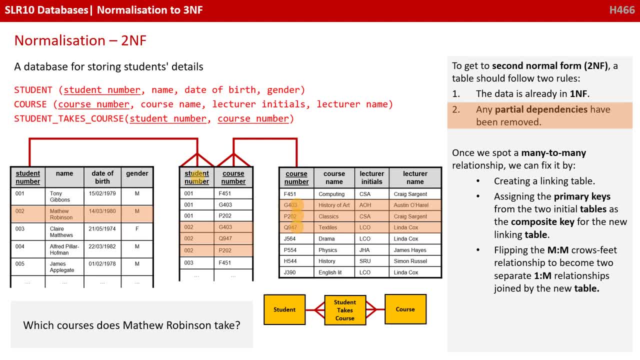 But that's OK because student number in the linking table is not unique. It's the combination of student number and course number that's unique And I can follow those records off to the final table to discover what courses he is covering. And I can do the same in the other direction Which students take computing. 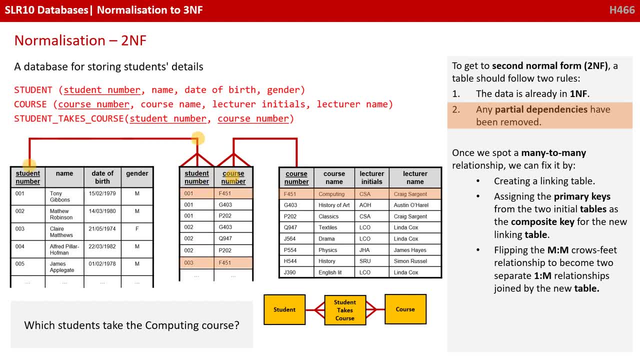 Well, I've got F451.. I go back into my linking table Now. F451 is not unique, but the combination of student and course number is. I discover two. I follow that back and I can tell you that Tony and Claire are taking computing. 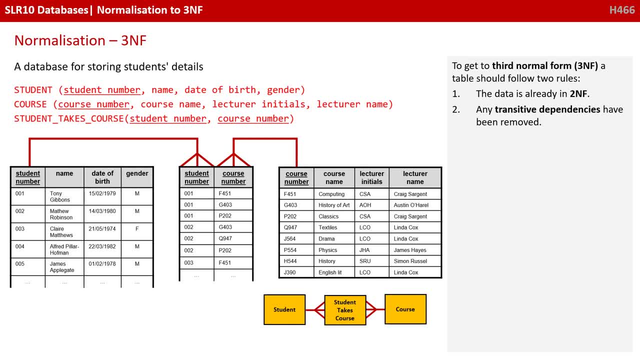 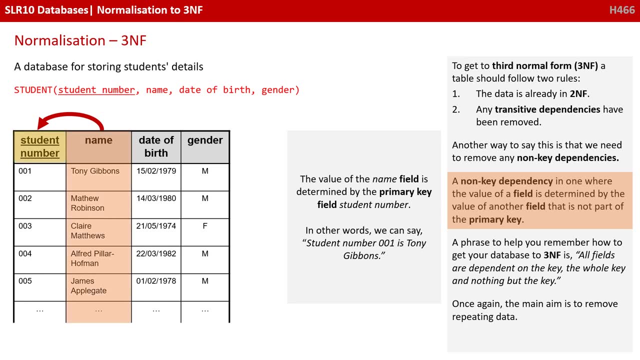 So now all we need is to get to third normal form. So again, two rules. The data is already in second normal form And are any transitive dependencies still around And have I removed them? So, just like with second normal form, where you had to get your head around partial dependencies, 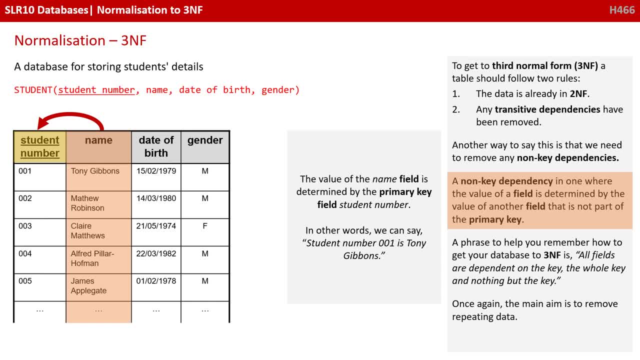 to really understand. third, normal form: you have to get what we mean by transitive dependencies. Another way to say this is that we need to remove any non-key- Non-key dependencies. A non-key dependency is one where the value of a field is determined by the value of another field that isn't the primary key. 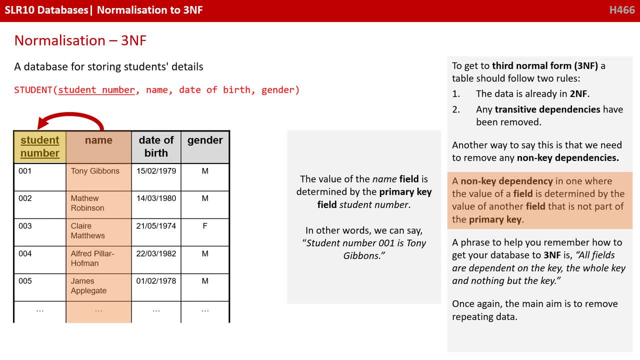 A nice phrase to help you remember how to get your database into third. normal form is: all fields are dependent on the key, the whole key and nothing but the key. Now, the overall aim here again is to remove repeating data, So let's start with the name field. 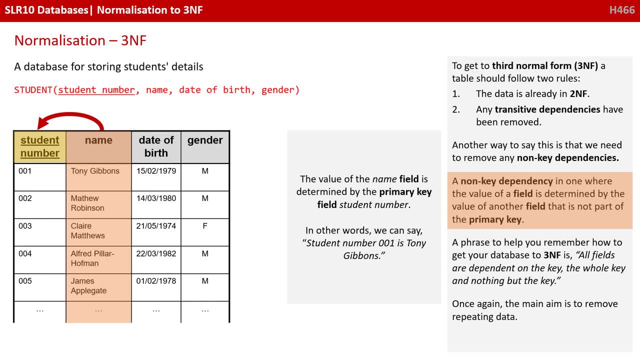 The value of the name field is determined by the primary key field: student number. In other words, we can say student one is Tony Gibbons. So the name field is dependent on the key, the whole key and nothing but the key. Now let's look at date of birth. 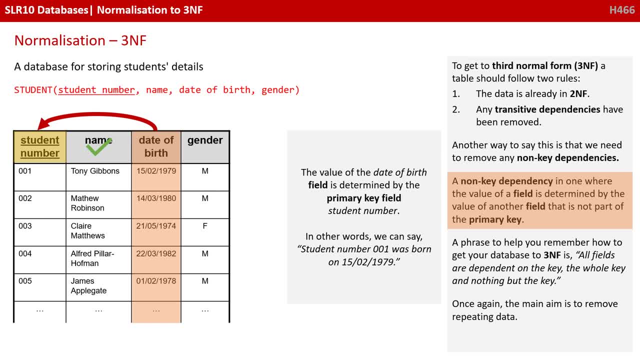 The value of the date of birth field is determined by the primary key: student number. In other words, we can say Student one was born on the 15th of the 2nd 1979.. Date of birth is dependent on the key, the whole key and nothing but the key. 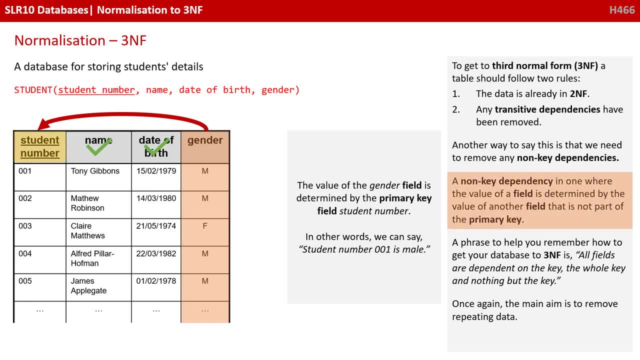 Looking good so far. Now we say the value of the gender field is determined by the primary key. In other words, we can say student 001 is male. The gender field is dependent on the key, the whole key and nothing but the key. 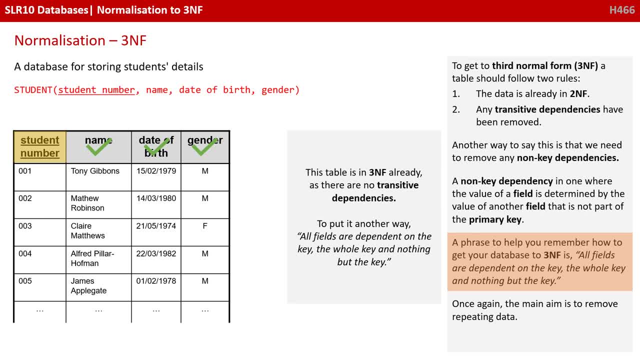 So what we've discovered is this table is already in third normal form. There are no transitive dependencies, Or, to put it another way, all the fields are dependent on the key, the whole key and nothing but the key. So this table is already in third normal form. 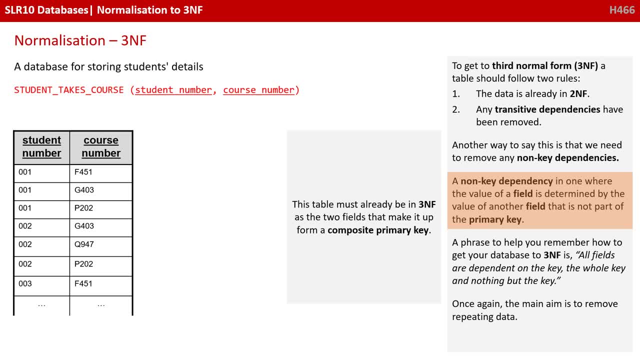 OK, the other table we've got is this linking table. Now, this table must already be in third normal form, As it only has two fields, and together they make the composite key. So that's great. OK, let's move on to our last table. 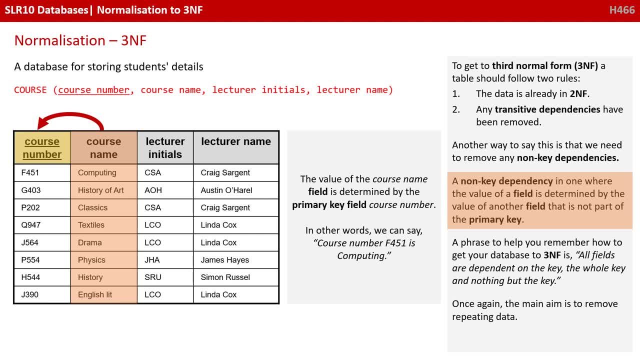 And again, let's look at each field in turn. So the value of course name is determined by the course number. In other words, we can say: course F451 is computing. Course name is dependent on the key, the whole key and nothing but the key. 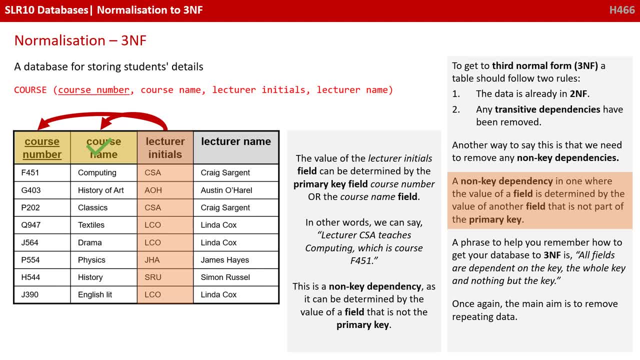 The value of the lecturer's initials field can be determined by the primary key or the course name field. So here we've hit our issue. In other words, we can say: lecturer CSA teaches computing, which is also course F451.. This is a non-key dependency, as we can determine this key by a value which isn't the primary key. 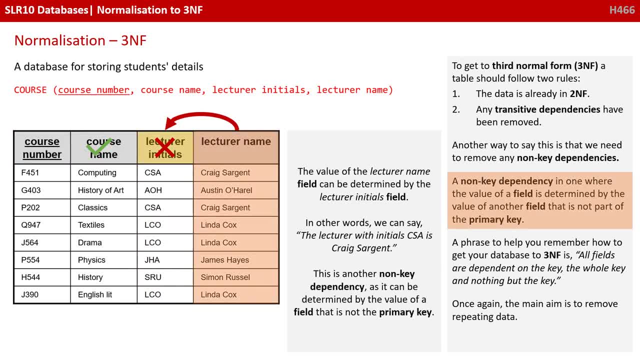 OK, let's look at our last field. So we've got the value of lecturer name field can be determined by the lecturer's initials. In other words, we can say the lecturer of initials CSA is Craig Sargent. This is another non-key dependency, as it can be determined by the value of a field that's not the primary key. 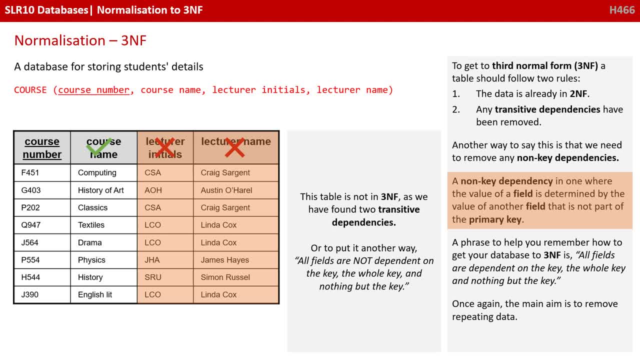 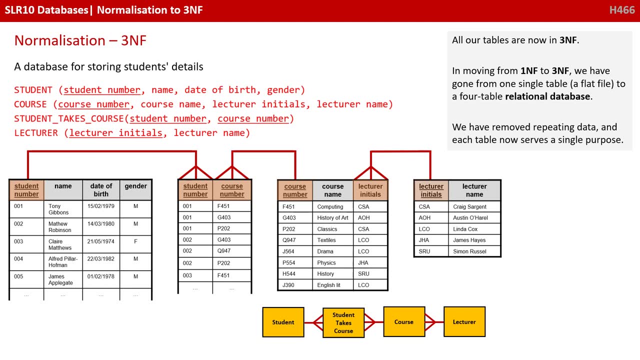 This table is not in third normal form, As we found two Transitive dependencies. or, to put it another way, all fields are not dependent on the key, the whole key and nothing but the key. We've now split those two fields apart and created a one to many relationship. 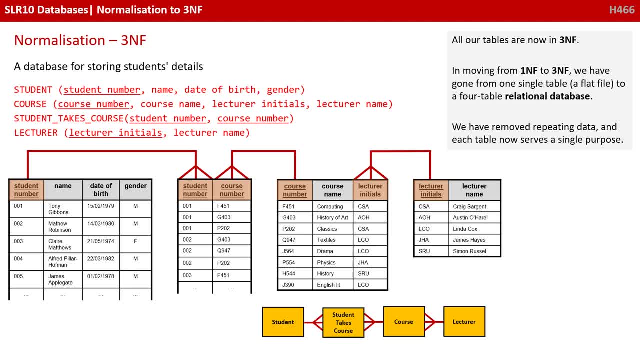 All our tables are now in third normal form. In moving from first to third normal form, We've gone from one single table, a flat file, To four tables in a relational database. We've removed lots of repeating data and each table now serves a single purpose. 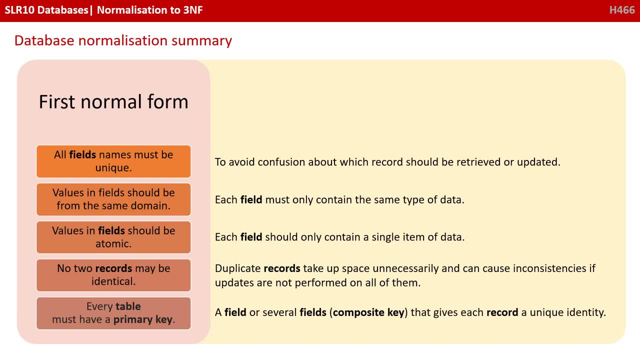 OK, so that was probably quite a lot to take in If you're looking to take some notes on this video, the next few slides being designed to help you bring that stuff together. So on the left we have here The five rules for first, normal form. 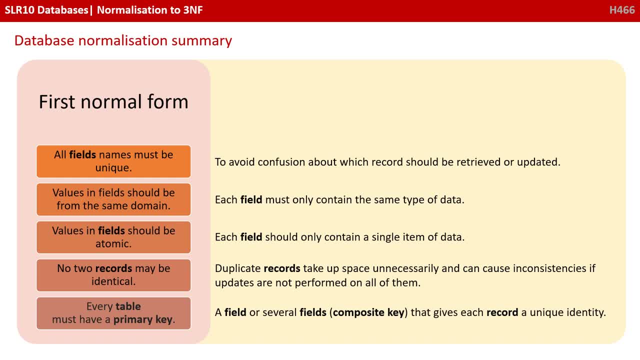 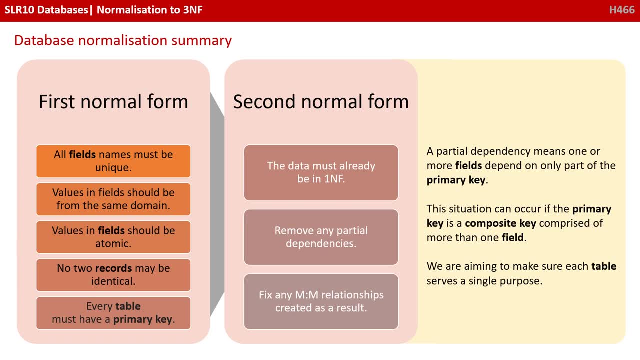 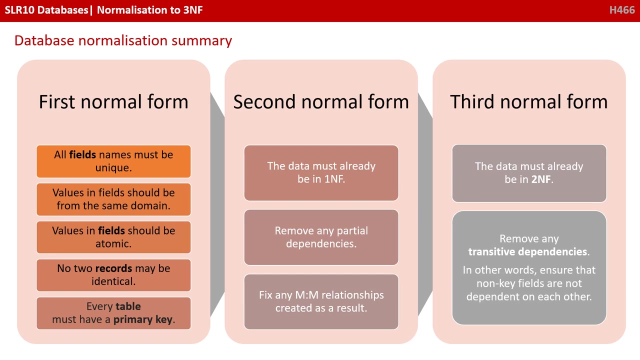 And on the right we have a bit of explanation of what some of those rules means. Pause the video and take some notes. Here we have the rules for second normal form, Again along with a few extra explanation notes, And finally we have the rules for third normal form. 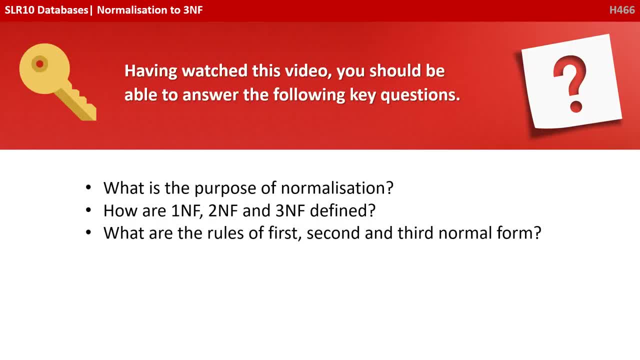 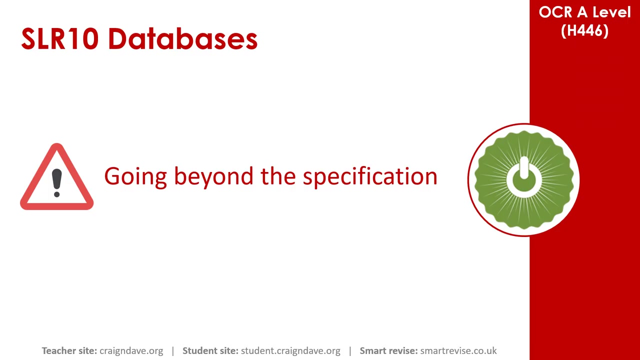 So, having watched this video, you should be able to answer the following key questions: What is the purpose of normalization, How are first, second and third normal form defined, And what are the rules of first, second and third normal form? OK, you can definitely put your pens down at this point. 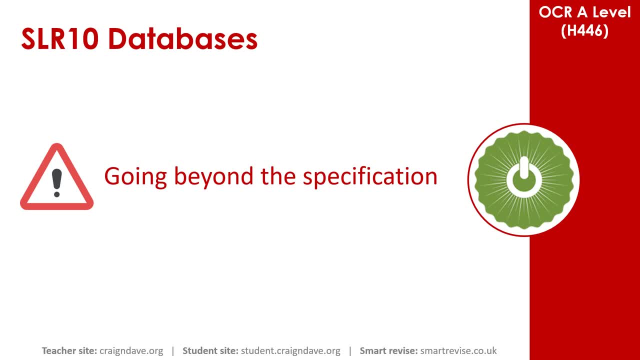 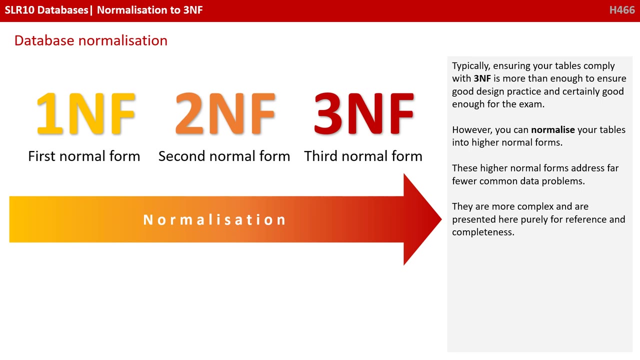 But if you want to know a little bit more about normalization that goes beyond that, Carry on and watch the last final bit of this video. You made it this far. You might as well. So typically, ensuring your tables comply with third normal form is more than enough to ensure good design practice. 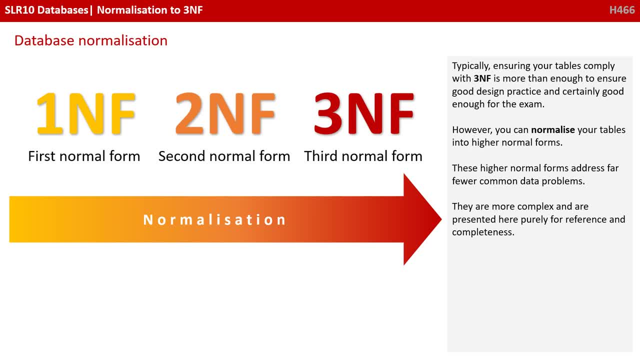 And it's certainly good enough for your exam. However, you can normalize your tables into higher normal forms. These higher normal forms address far fewer common data problems. They're more complex and they're presented here purely for reference and completeness. So after third normal form, we have Boyce-Codd normal form. 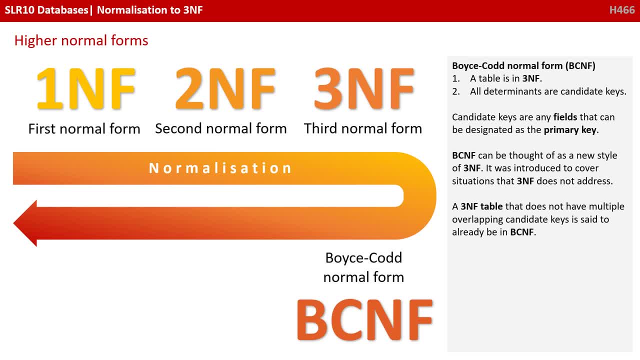 A table is in BCNF if it's in 3NF and all determinants are candidate keys. Now, candidate keys are any fields that can be designated as the primary key. BCNF can be thought of as a kind of new style of 3NF. 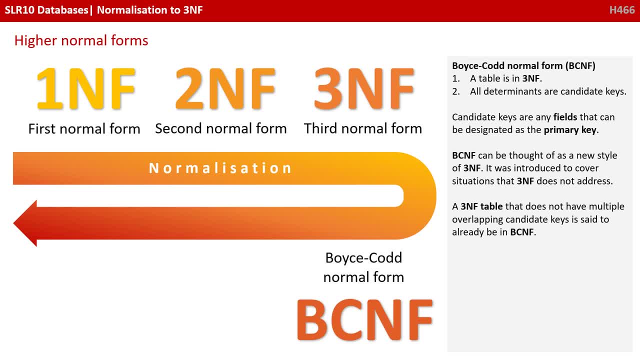 And it was introduced to cover situations, To cover situations that 3NF didn't address. A 3NF table that does not have multiple overlapping candidate keys is already said to be in BCNF. Beyond that we have fourth normal form. That's a table that's in BCNF and there are no multivalued dependencies. 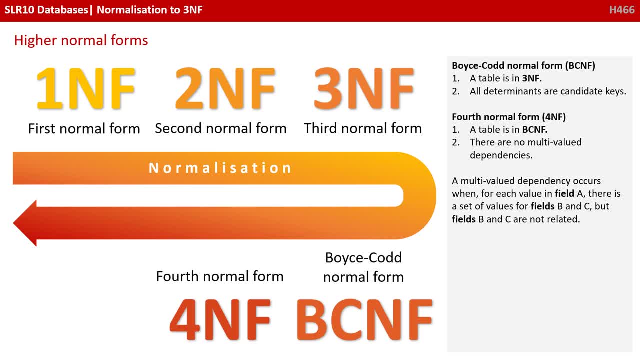 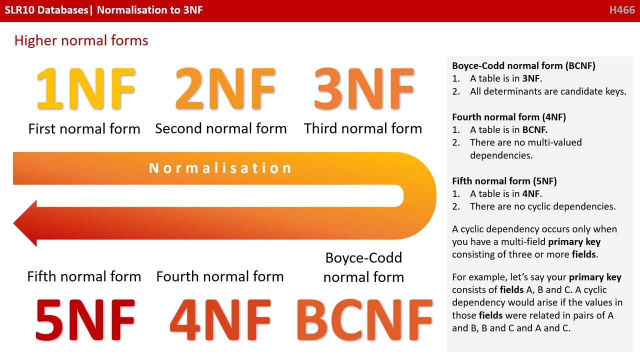 A multivalued dependency occurs when for each field in field F there's a set of values for field B and C, But B and C are not related to each other. And finally, we have fifth normal form. That happens when a table is in fourth normal form and there are no cyclic dependencies. 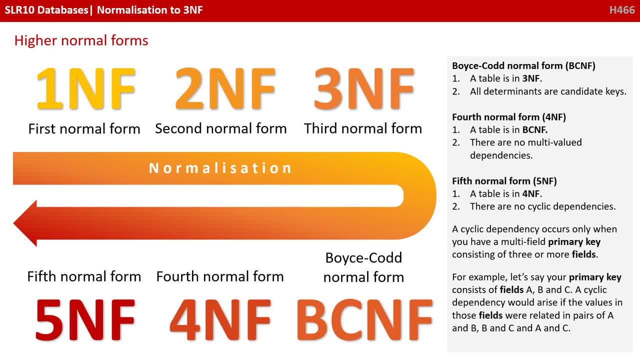 A cyclic dependency occurs only when you have multi-field primary keys consisting of three or more fields. So, for example, we could say a primary key consists of fields A, B and C. A cyclic dependency would arise if the value of those fields were related in pairs of A, B, B, C and A- C. 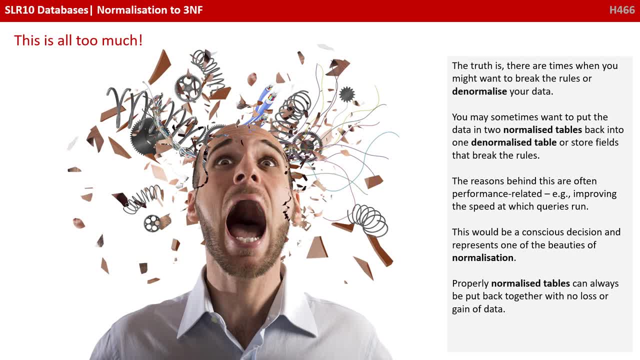 OK, so it's got all too much. Well, there's a bit of a truth here about database normalization. There are times when you might actually want to break the rules or denormalize your table. So don't panic. You may sometimes want to put data in two normalized tables back into one. 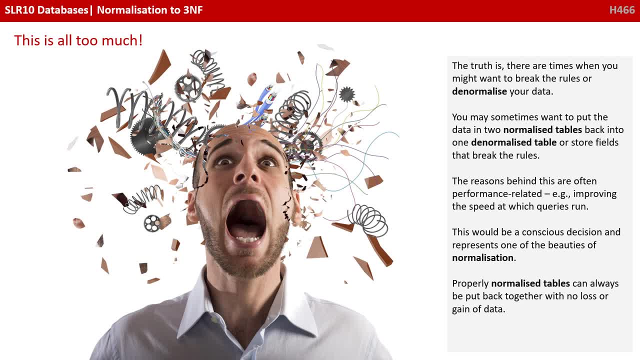 Denormalize table or store fields that break the rules, And the reason behind this are often related to performance. The whole point of normalization is to improve the speed at which queries are run, But of course, this would be a conscious decision and represent one of the beauties of normalization. 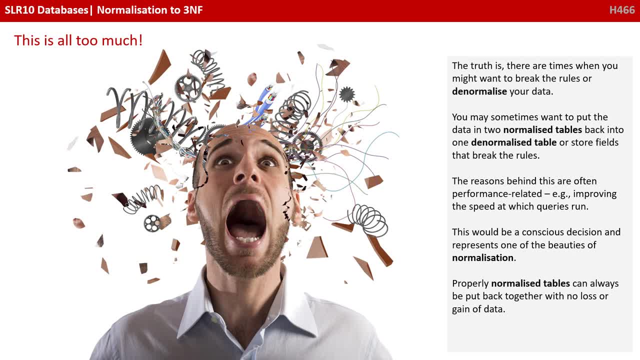 because if you've properly normalized tables, you can always put them back together with no loss or gain of data. We've got one more video after this, which provides another step by step example of how to normalize a database to third normal form. So we haven't got this yet. Take a break. 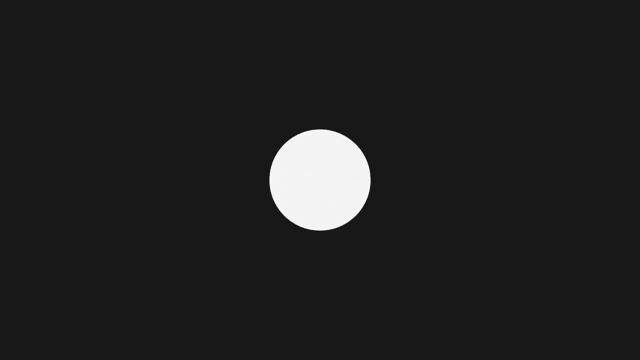 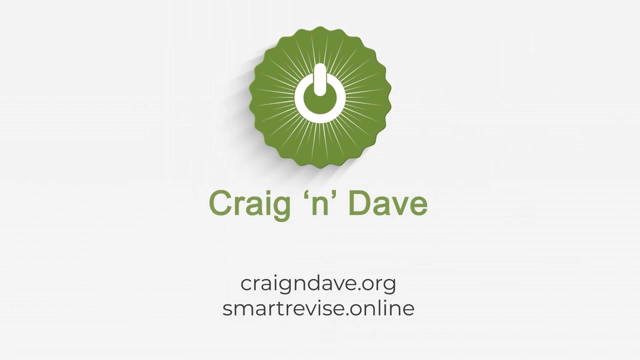 Come back and watch that one. Thanks for watching.